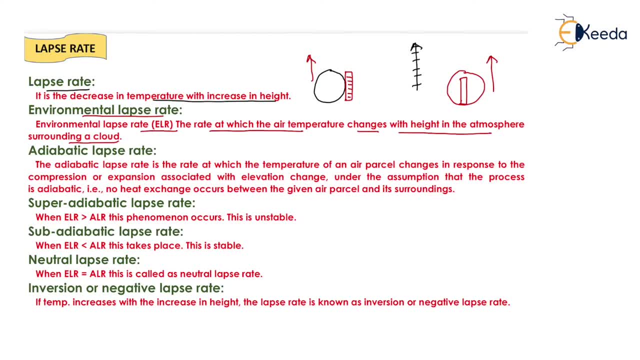 increase in altitude, the decrease in temperature of the inside environment of the balloon will be measured by this thermometer, and this decrease in temperature of the inside of the balloon is known as adiabatic lapse rate. now, the adiabatic lapse rate is the rate at which the temperature of an 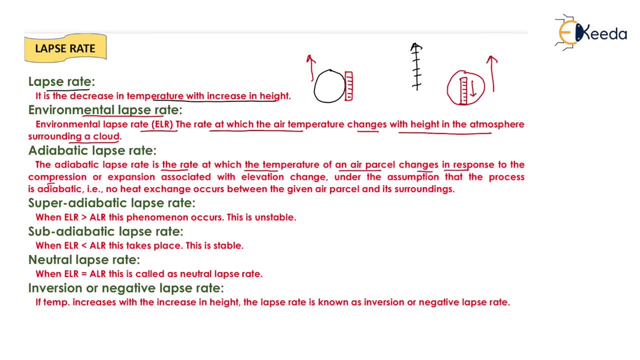 air parcel changes in response to the temperature of the balloon and the temperature of the air response to the compression or expansion associated with elevation change. under the assumption that the process is adiabatic, that no heat exchange occurs between the given air parcel and its surrounding, okay now, depending on the environmental lapse rate and adiabatic lapse rate. 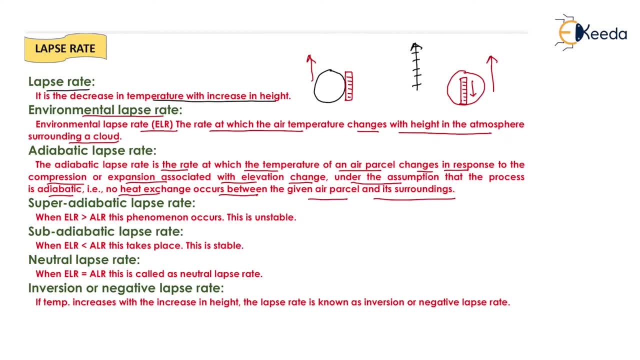 we had three types of condition, that is, super adiabatic lapse rate, sub adiabatic lapse rate and neutral lapse rate. when the decrease in temperature of the outside environment is greater than the decrease in temperature of the inside of that here, inside of the of that air balloon, then that 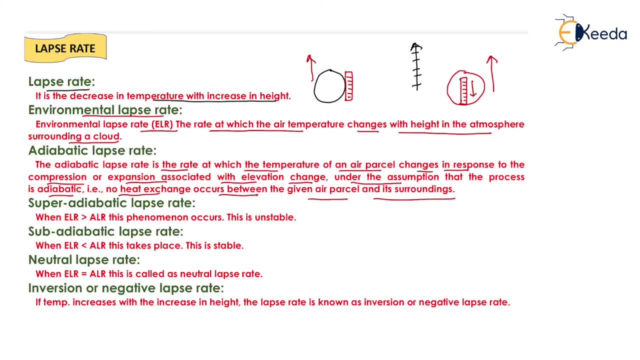 type of lapse rate is known as super adiabatic lapse rate. it means that when environmental lapse rate is greater than the adiabatic lapse rate, it means that when the decrease in temperature of the outside environment is greater than the decrease in temperature of the inside of air balloon, then 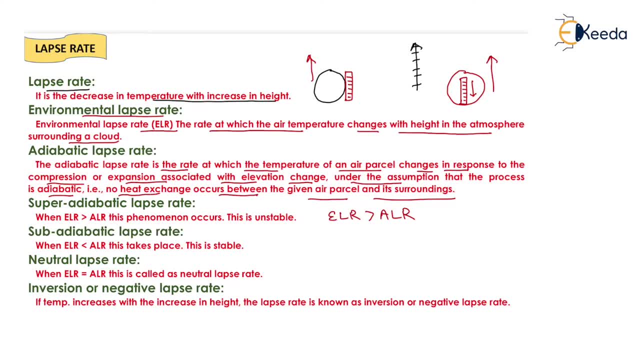 that phenomena is known as super adiabatic lapse rate, and it is an unstable state. okay now next one is the sub adiabatic lapse rate. when ELR, that is, the environmental lapse rate, is less than the adiabatic lapse rate, it means that the decrease in temperature of the outside environment is less than the 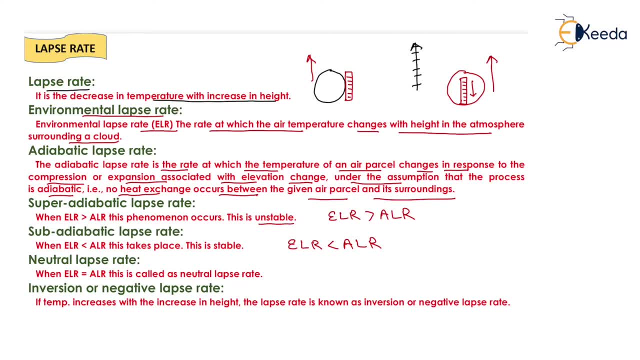 decrease in temperature of the inside of air balloon. then that type of lapse rate is known as sub adiabatic lapse rate and it is a stable state. when the environmental lapse rate will be equals to adiabatic lapse rate, then this state is known as neutral lapse rate. okay, now at the higher. 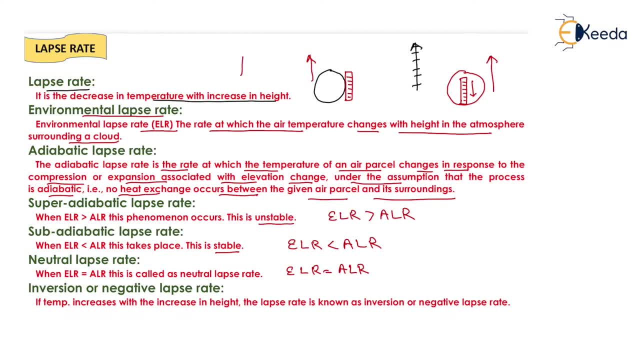 atmosphere. what will happen? with increase in the height, the increase in temperature will takes place, okay, at the very high altitude of the atmosphere. with increase in altitude, the increase in temperature will takes place. now, if temperature increases with the increase in height, the lapse rate is known as inversion or negative lapse rate. that is all about the dispersion of air.